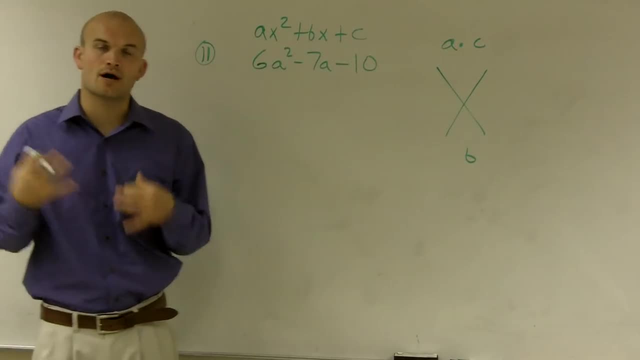 Alright, if you guys can see, Kind of remember this. This is the very way, like foolproof way, to always check. So I do: 8 times c, 6 times negative 10,, which would be a negative 60,. 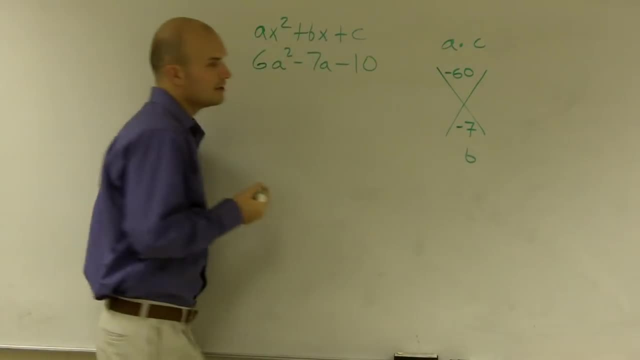 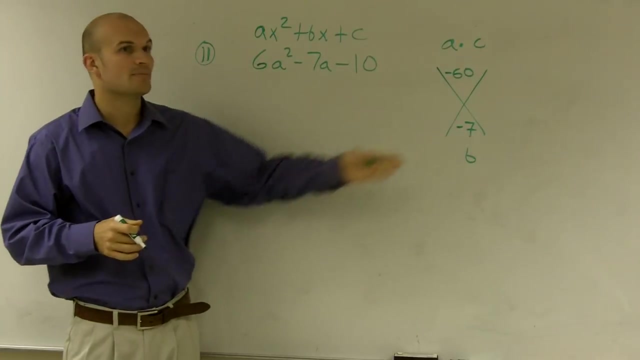 and then my b is a negative 7.. Alright, so then I need to look at this and I see: alright, what two numbers multiply to give me a negative 60, but then add to give me a negative 7? So you can look at all the factors of negative 60.. 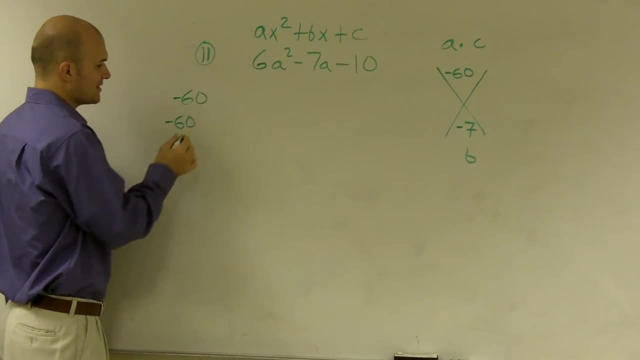 Alright, you could have negative. well, it's going to be a negative 60. So it would be negative 60 and 1, or it could be negative 1 and 60, right, But I'm just going to do one set. So you could do negative 6 times 10.. 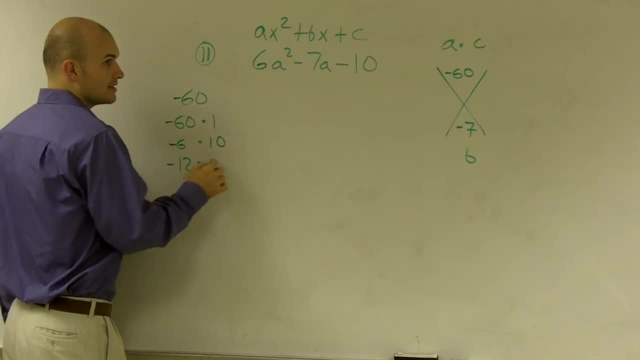 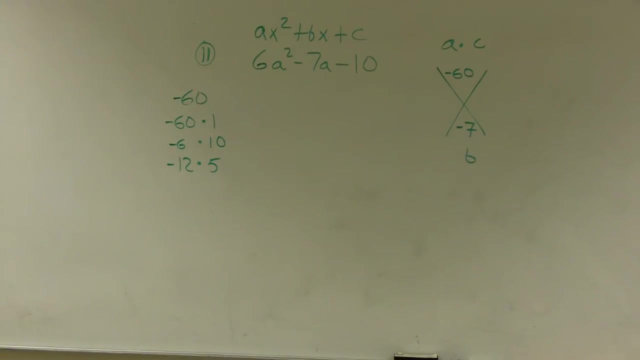 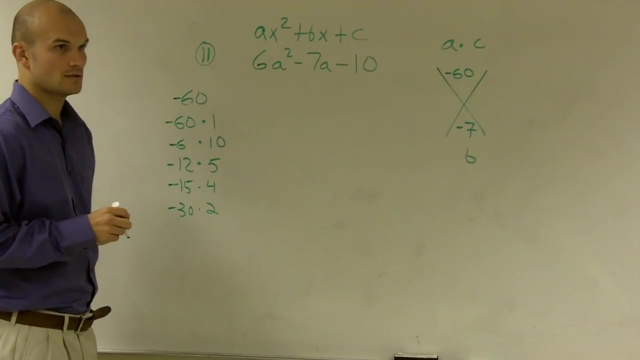 You could do negative 12 times 5.. I'll hide it here, Okay, thank you. You could do negative 15.. One, four negative 30 and 2, and 12 and 5, and you could do negative 3 and 20,, right. 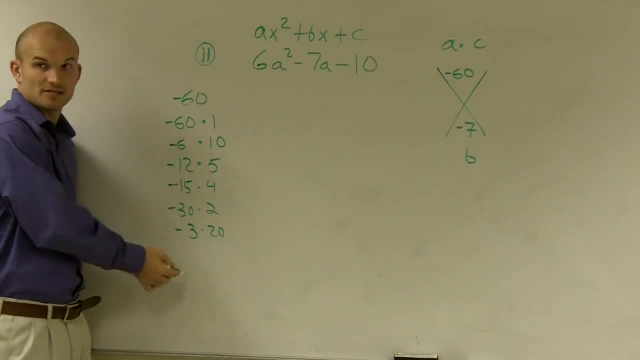 Now, obviously you could all- I could- swap these right. These could all be negative and these could be positive, right? So there's a lot of possibilities. However, just look at the numbers. What numbers have a difference of 7?? 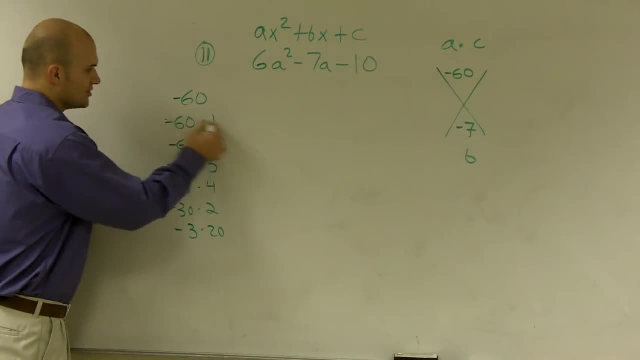 And don't worry about the numbers Plus or minus. But what numbers have a difference of 7?? Those don't. Those have a difference of 4.. Those have a difference of 11.. Difference of 18.. Difference of 17.. 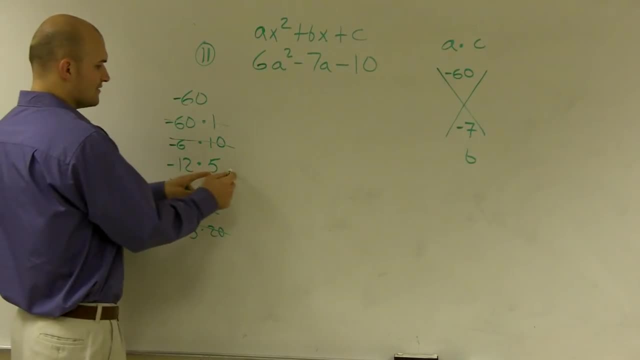 But you can see these two have a difference of 7, right. So it either could be negative 7 and 5, or 12 and negative 5, right. Well, 12 times When you look at this, which two of these added up give me negative 7?. 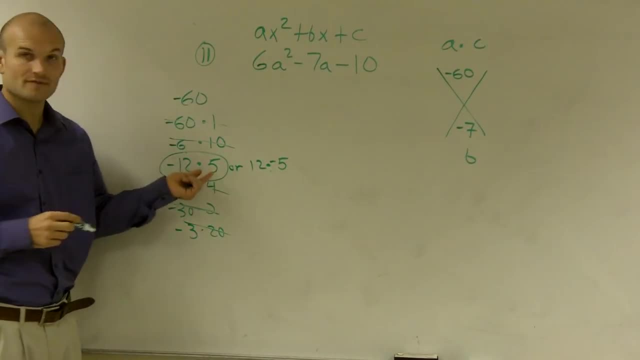 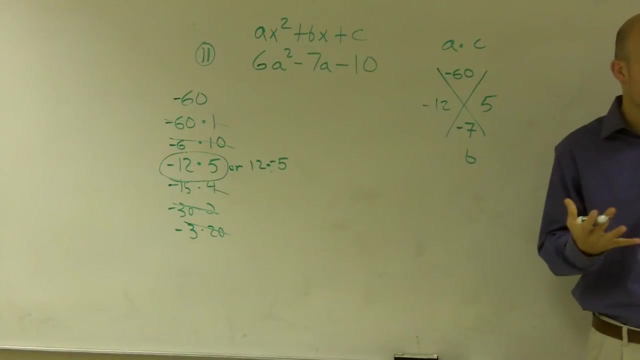 And yes, That is my solution: Negative, 12 and 5.. So I can write negative 12 and 5, right. Now. everybody's so used to always saying, oh, these are your two answers: x minus 12 and x plus 5, right. 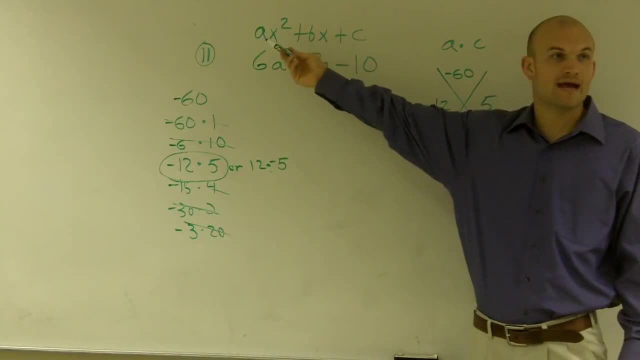 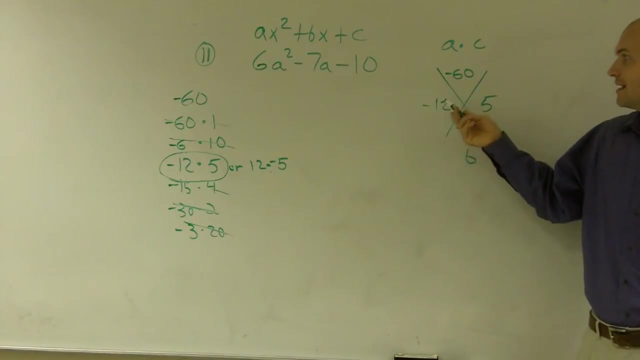 That's when everybody gets mixed up, because before, when we solved, when their a was 1, that's what we did. We just took these two numbers and we said x minus 12 and x. you know, x plus 5.. The problem with that is x times x does not give you a 6a squared. 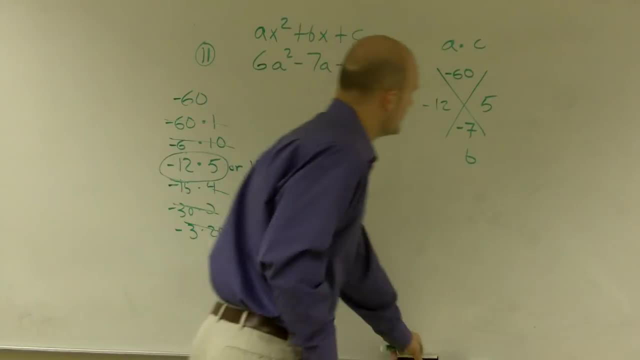 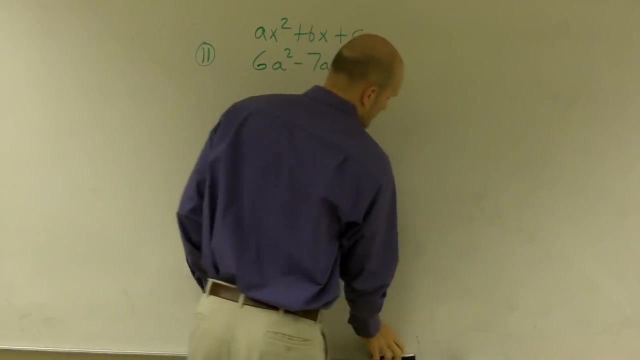 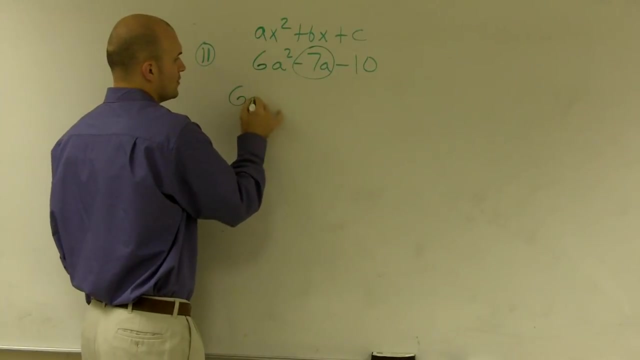 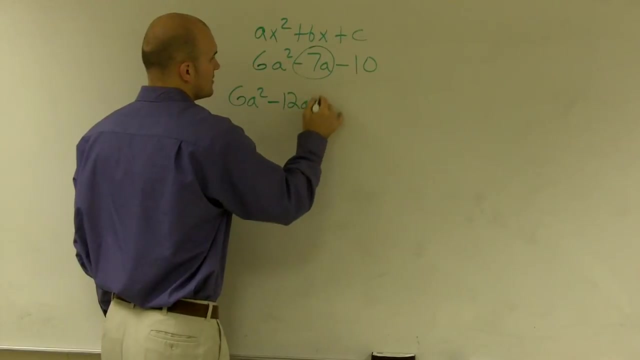 So there's a couple ways we could do this, And I'll do it two different ways, And you guys can determine which way is confusing and which way makes sense. OK, One way is we can rewrite this formula with a. what was it? a 12a plus 5a minus 10.. 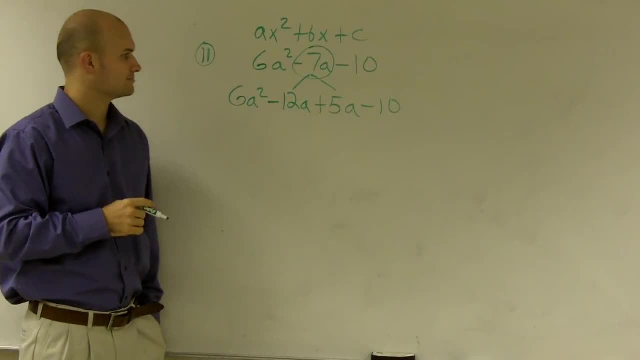 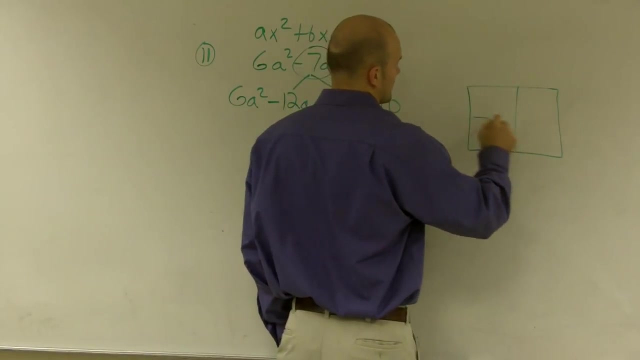 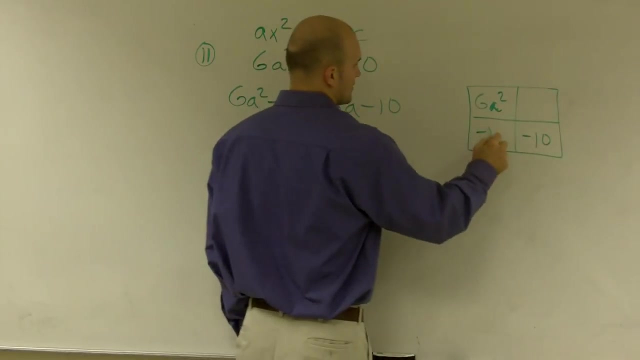 So, instead of writing a negative 7a, we could write it like this: All right, The other way you could do it is what we call the box method. You take your a, which is 6a squared, You take your c, which is negative 10, negative 12a and plus 5a. 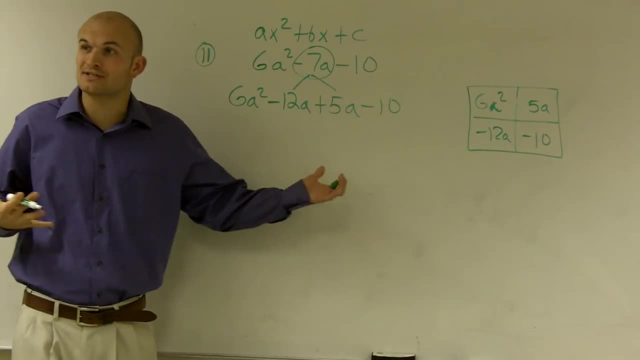 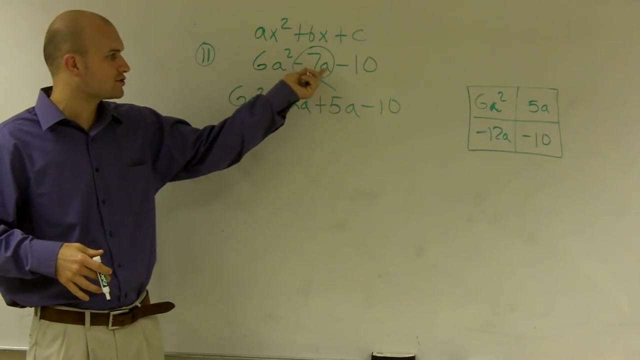 OK, So there's two different ways. we can kind of do this. You're really doing essentially the same thing. This is a way just to organize it. This is a way just to organize it differently. Well, all I did was I rewrote my middle term as two different ways. 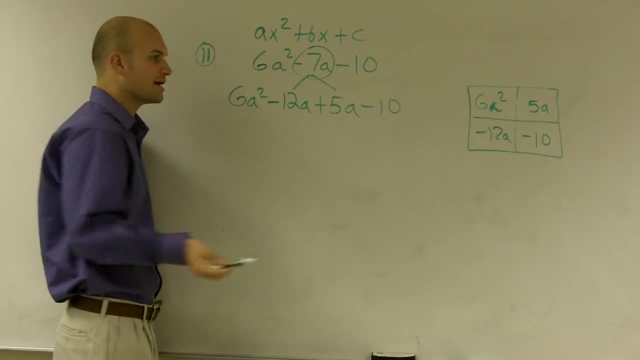 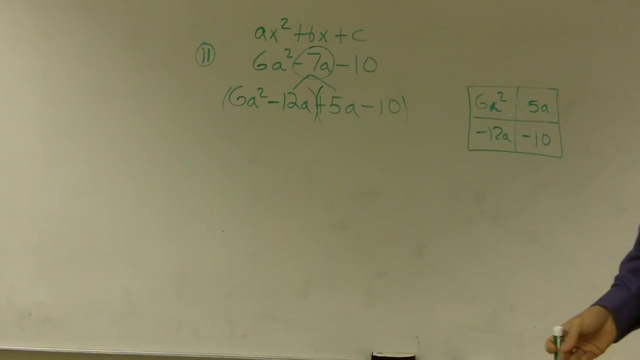 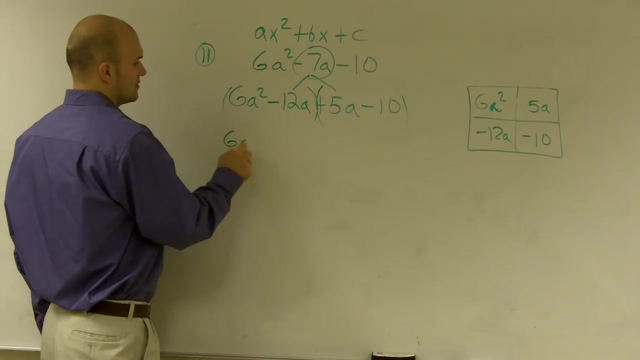 So one way I could do- for this way, the reason why I'm doing this- is factor by grouping right: Group the first two terms, Group the first two terms and say what can I take out of here? And you could say: well, you could factor out a 6a right. 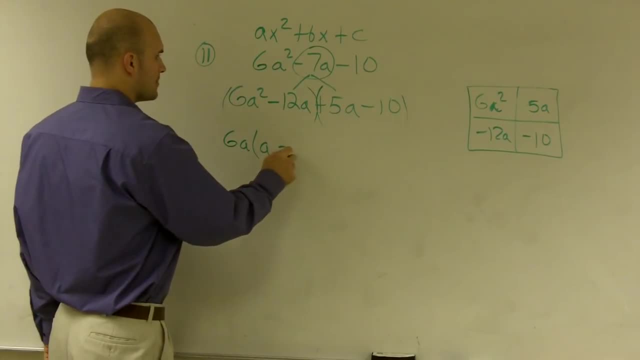 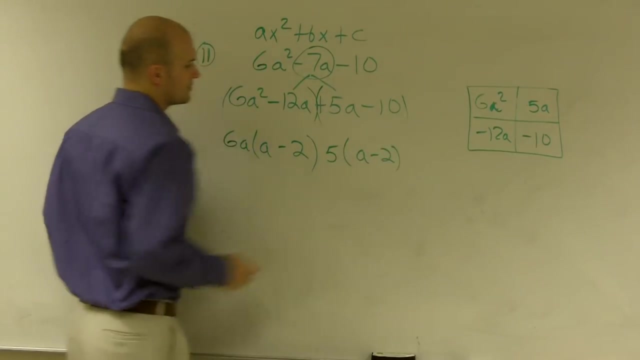 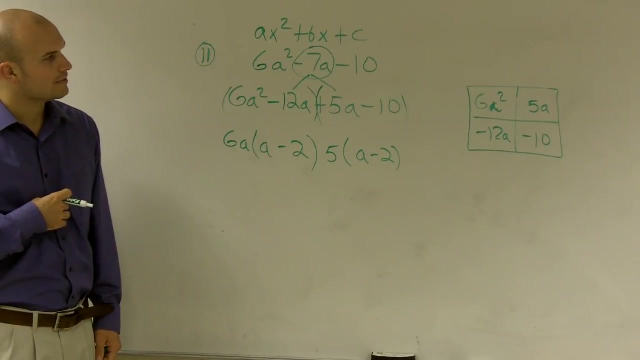 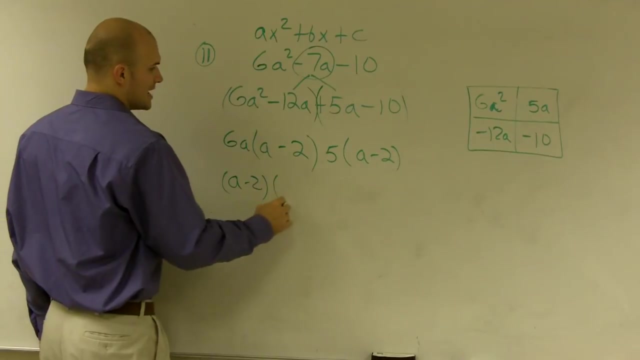 6a, left with a minus 2.. Minus 2.. Then here I can factor out a 5. And I'm left with a minus 2.. Right, And then let's see here. Then from here you can factor out an a minus 2 times a 6a minus 5.. 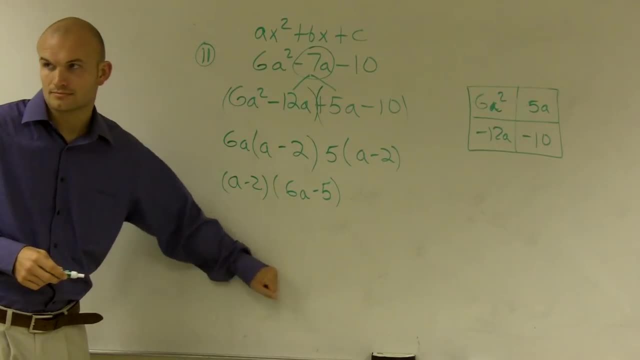 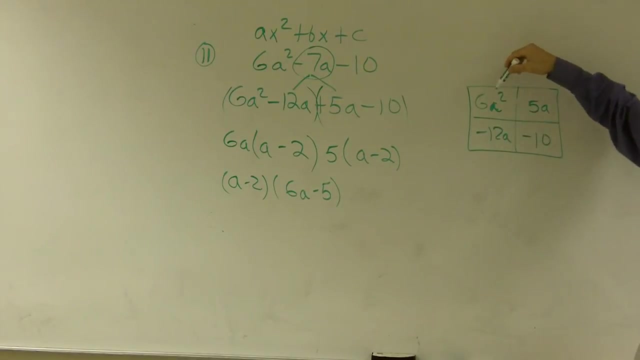 So that would be your two factors. OK, Over here. how do I solve it from here? Well, it's pretty much the exact same thing. Remember, when you're doing the box, you want to say what two numbers multiply to give me what's inside my box. 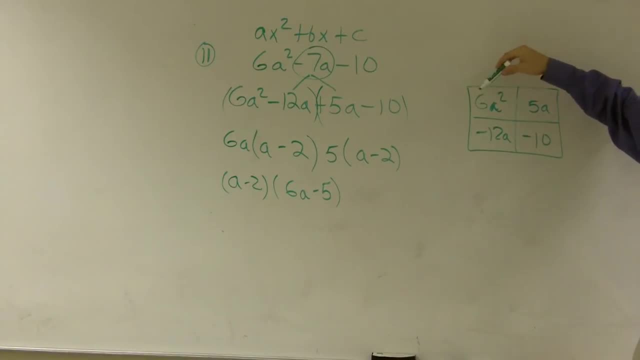 So what two numbers multiply to give me 6a times 2?. Now, easily you could say: well, 3 and 2 work right. Well, if I put a 2 there 2 times, what gives you 5?? 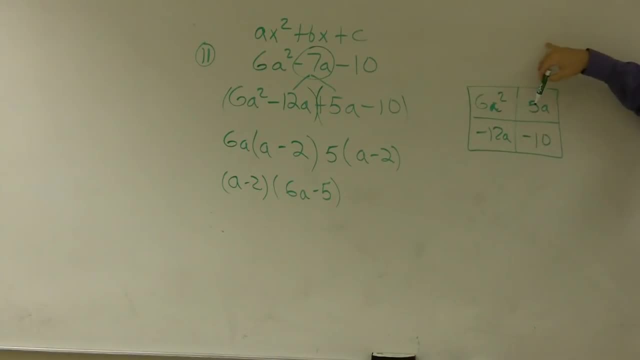 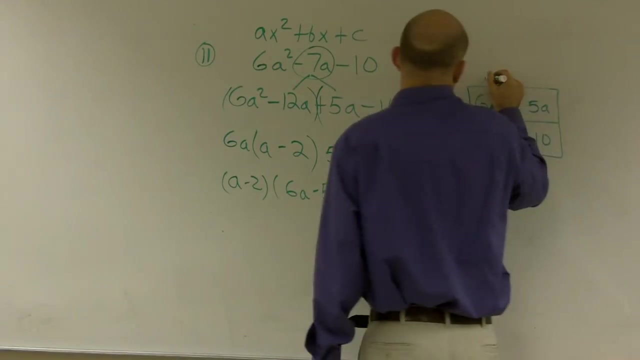 That's going to be a fraction, right? What if I put a 3 there, 3 times? a fraction is going to give you 5,, right? So we're going to have to come up with new numbers. How about if we did 6a? 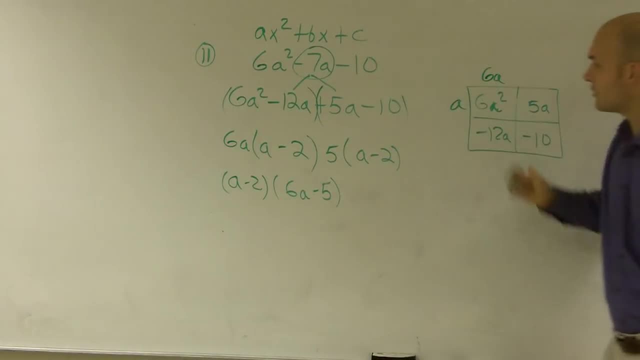 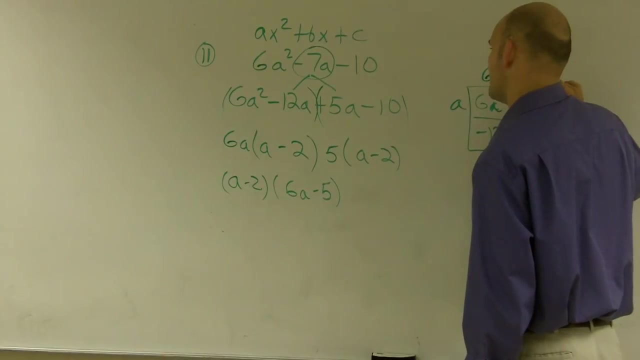 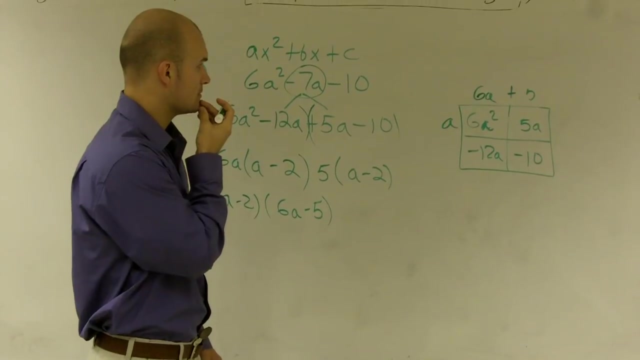 6a times a. Well, that will work, because a times what gives you 5a 5, right, That's a negative. That's what, When you multiply negative 5 and negative 2 together, it doesn't equal negative 8.. 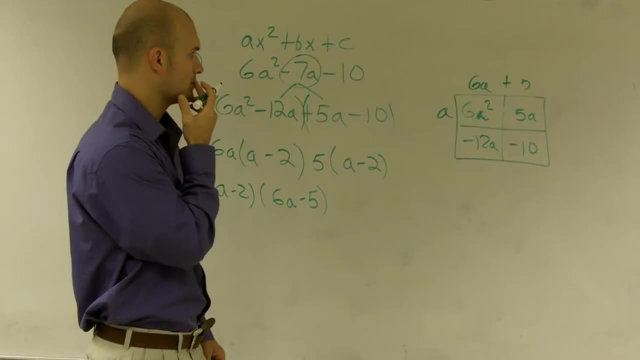 I mean negative 10 equals positive 10.. Where did you get the positive 10?? So it's got to be a plus 5 and then a minus 2.. Are you talking about in here? Yes, Yeah, it was supposed to be a plus 5.. 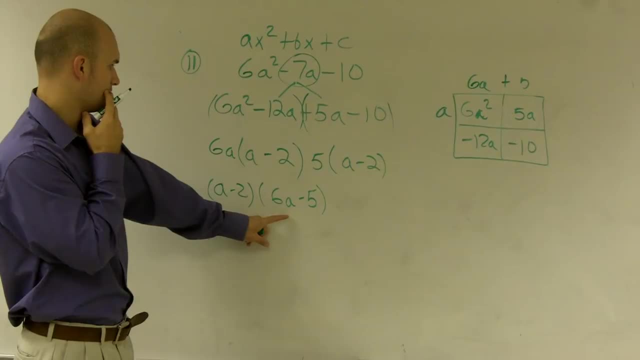 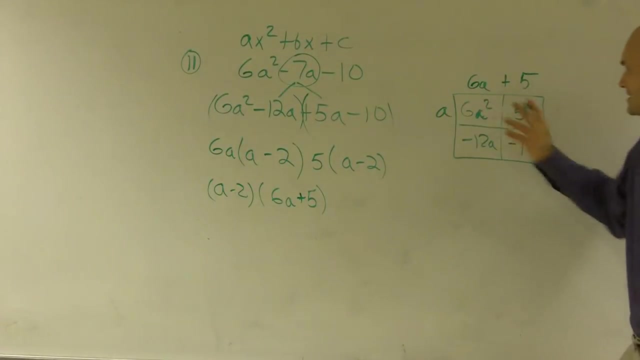 Where did I miss that? Right by your finger? Oh, that's a plus 5.. Yes, thank you. Yeah, 6a, that's plus 5.. Thank you Because that makes sense, because a times what gives you 5a?